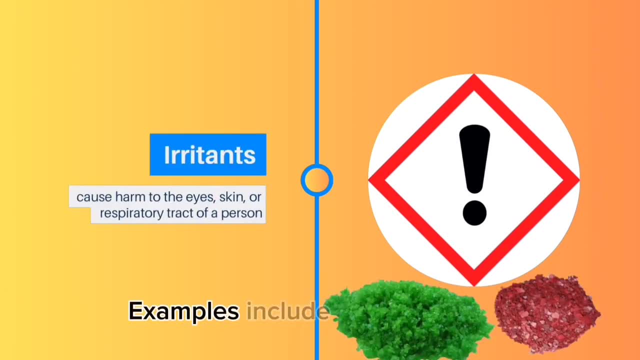 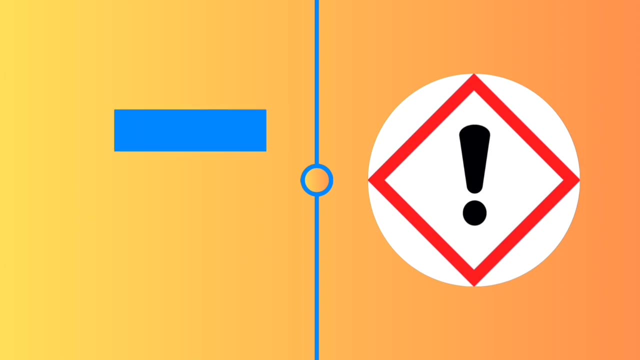 with long-lasting health impacts or even be fatal. Examples include nickel chloride, chromic acid Sensitizers. Sensitizers are also known as allergens, meaning they cause an allergic reaction in people who face repeated exposure over time to certain chemicals. Reactions to 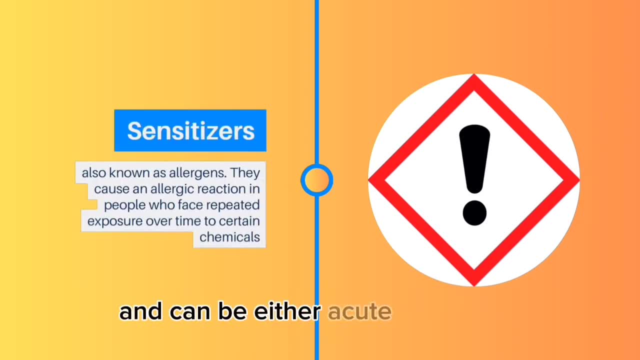 chemicals deemed as sensitizers are often called allergens. Sensitizers are also known as allergens. Sensitizers vary from person to person and can be either acute or chronic. Chemical exposure can manifest as swelling of the airway or develop into dangerous illnesses such as lung disease. 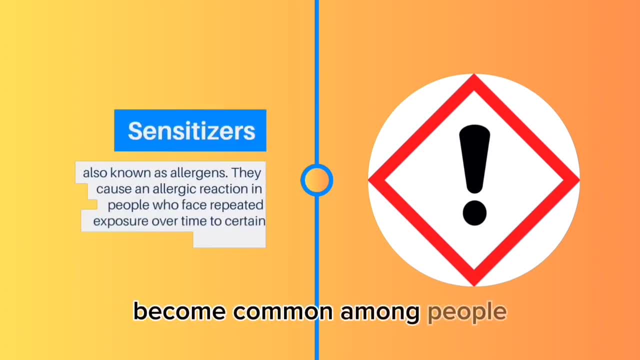 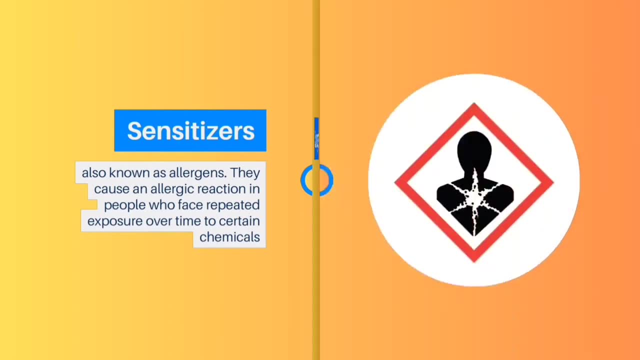 Some diseases, such as asthma and contact dermatitis, become common among people due to overexposure to chemicals. Examples include chlorine, alkalis, benzylic and allylic halides- Carcinogens. Carcinogens are cancer-causing chemical substances and a small amount of 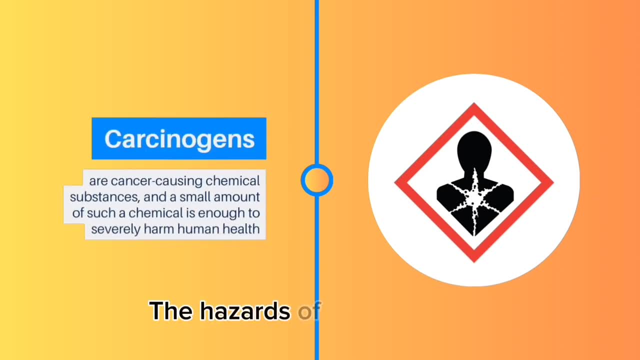 such a chemical is enough to severely harm human health. The hazards of such chemical substances will only appear if the chemical is not used in the right way. Carcinogens are often used in the right way. Carcinogens are also used in the right way. Carcinogens are also used in the right way. 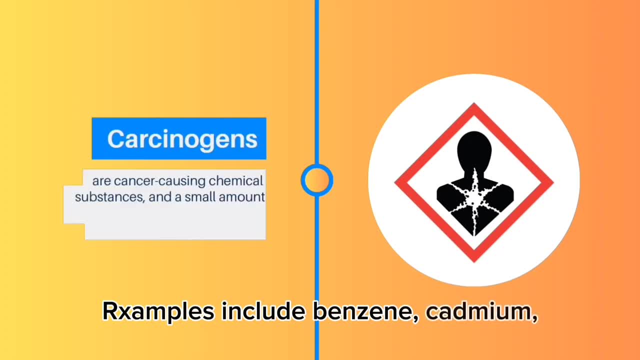 After exposure. Examples include benzene, cadmium, formaldehyde, vinyl chloride Mutagens. Chemicals classified as mutagens cause genetic changes to a cell's DNA and RNA. Genetic changes can cause cancer, prevent normal biological functions or may result in the. 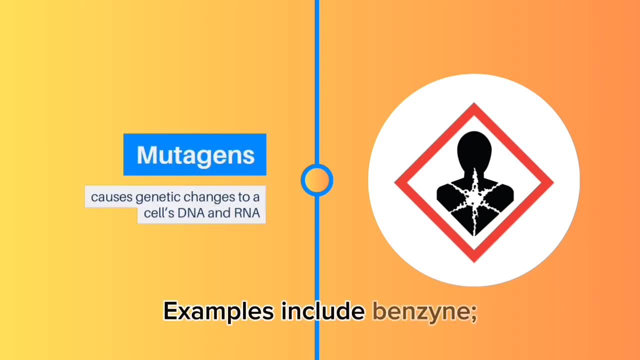 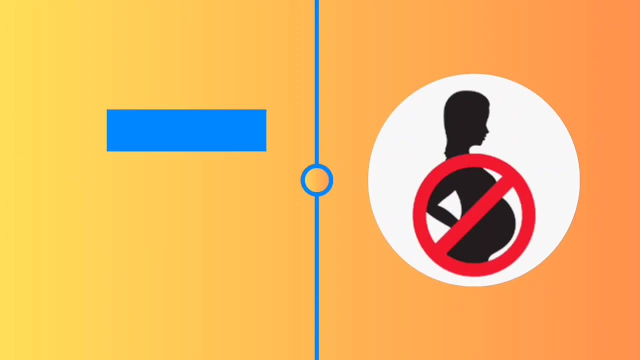 malfunction of a particular organ. Examples include benzene, Ionizing radiation, Teratogens. Chemical teratogens can disrupt the normal development of a fetus, causing birth defects and even the healthy advancement of the fetus. Carcinogens are also used in the right way. 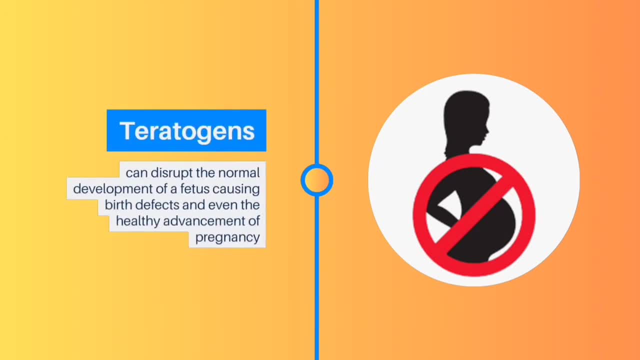 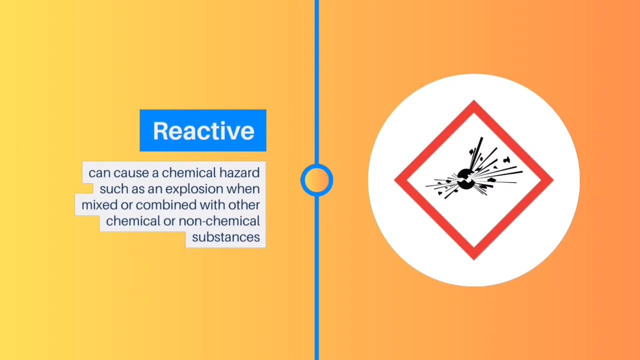 Pregnancy. Examples include thalidomide. Ionizing radiation, Organic mercury compounds. Reactive Chemical substances that cause a chemical hazard such as an explosion when mixed or combined with other chemical or non-chemical substances, such as water or air. Examples include nitric acid, Benzoyl peroxide. 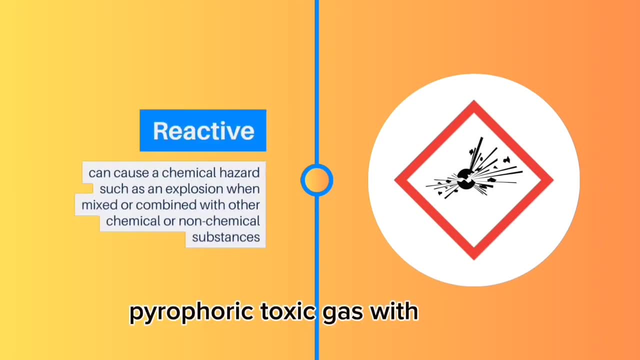 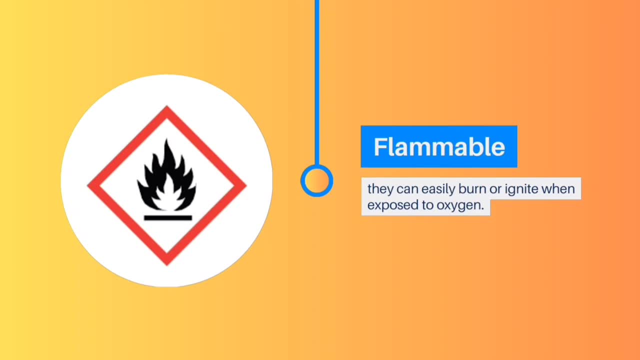 Silane. Silane is a colorless, pyrophoric toxic gas with a sharp, repulsive, pungent smell somewhat similar to that of acetic acid: Flammable. Many chemicals are characterized by a as flammable as they can easily burn or ignite when exposed to oxygen. Examples include methanol. 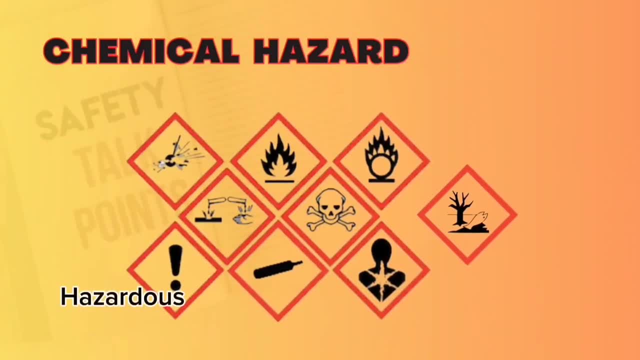 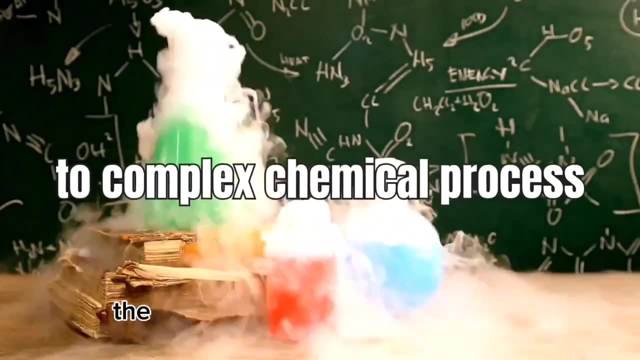 acetone, propane, butane. Hazardous substances are used for a variety of tasks, from simple cleaning operations to complex chemical processes. Hazardous substances have the potential to harm human health. They may be solids, liquids or gases. They may be naturally occurring.